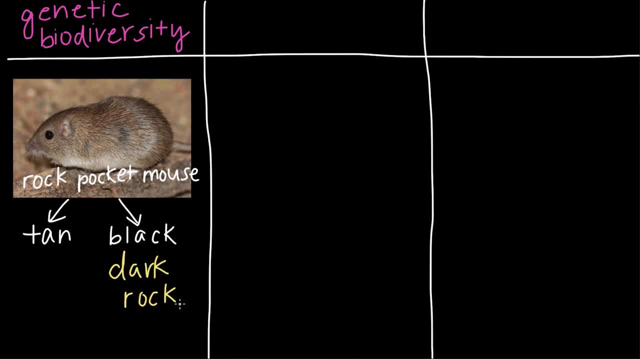 pocket mice in places with dark blackish lava rock, while there are more tan-colored rock. pocket mice in lighter colored sands Makes sense because, if you think about it, the mice are hunted from above by predators like birds. So having a coat color that blends into their surroundings would increase their chances of. 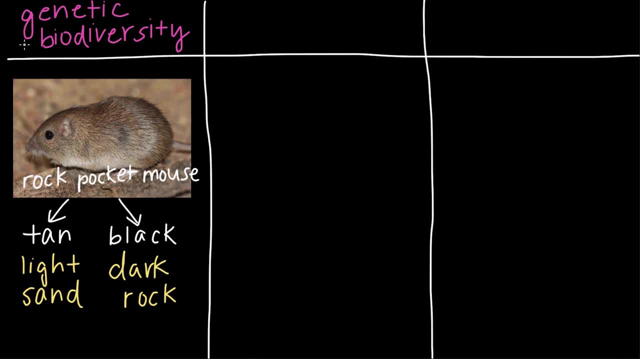 survival. So having this kind of genetic biodiversity is really great because the rock pocket mice can use many different colored landscapes as habitats And if, let's say, the landscape color were to change and suddenly become dominated by dark lava rock, then this population 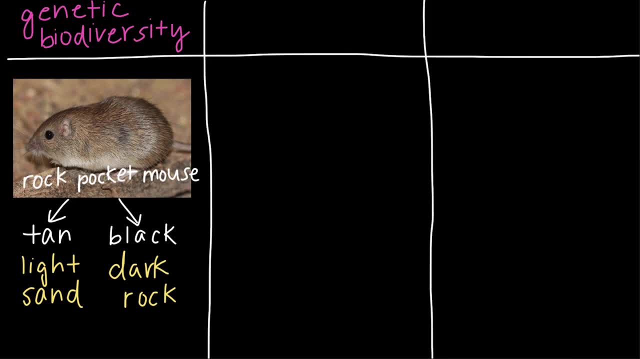 of mice would have the genetic diversity that it needs to adapt to this change. So the second level is species biodiversity, which is the variety of species in a particular area. So, going back to the Sonoran Desert, there are all kinds of mammals and birds, plants. 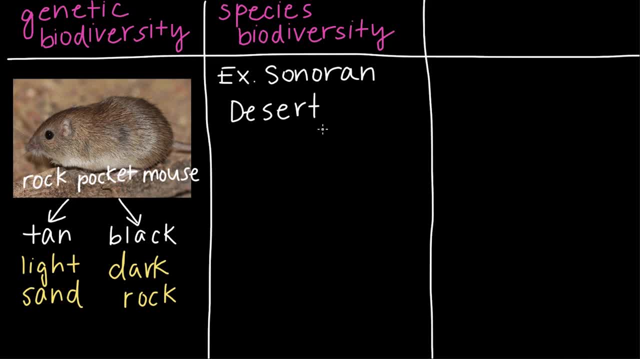 and insects. But what I think is even more mind-boggling is the sheer number of bat species there are. I mean, we have silver-haired bats, as I mentioned earlier, but also bats like spotted bats, western red bats and even this kind of bat called Peter's ghost-faced bat. 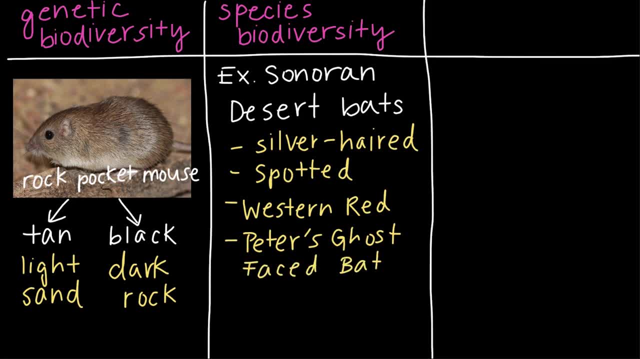 which I think is a really awesome name, And you're probably thinking: okay, Abby, this is really interesting, but so what? Well, like genetic biodiversity, species biodiversity is super, duper important, because having a lot of different species means that more roles can. 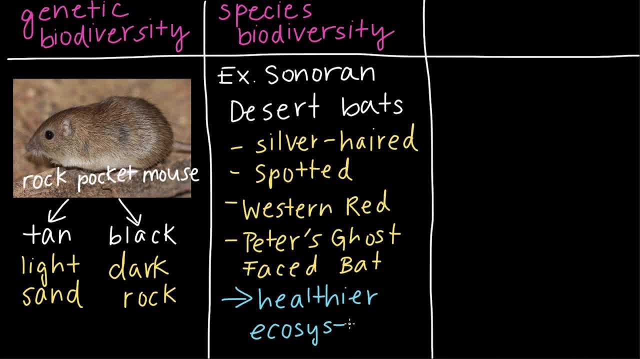 be filled in an ecosystem which makes the ecosystem healthier. So, moving on to the final level, we have. So, moving on to the final level, we have. So, moving on to the final level, we have ecosystem biodiversity, and this is just the variety of ecosystems on the planet. 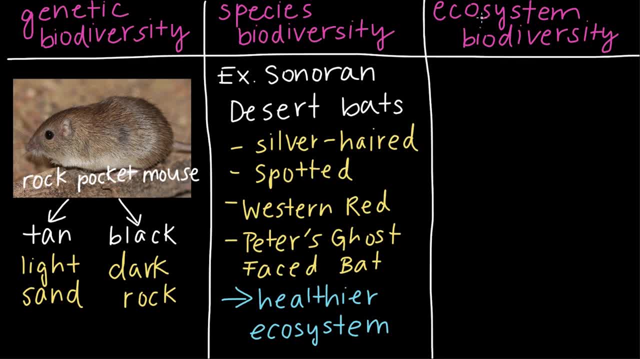 Now we've been talking a lot about the Sonoran Desert, and a desert is actually a type of ecosystem on Earth And, if you recall, ecosystems are made up of both living things and their physical environment. So in this case, living things in the desert ecosystem could include 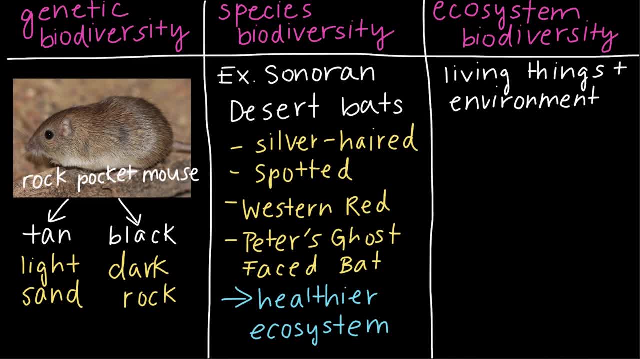 things like rattlesnakes, scorpions and cacti, while non-living things could include rock formations or sand dunes. And in addition to desert ecosystems, Earth has forest ecosystems, coral reef ecosystems, all kinds of different ecosystems. And having all these different kinds, 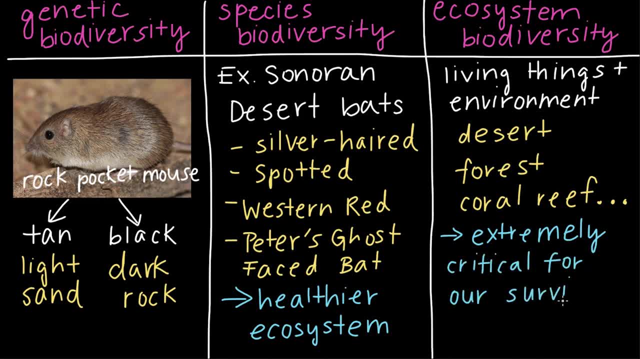 of ecosystems is extremely critical for our survival, because the diversity of ecosystems on Earth provide us humans with important resources and services. So without ecosystem biodiversity, our quality of life and, in fact, our very survival could be at risk. So, as you can tell, every level of biodiversity is incredibly important for unique. 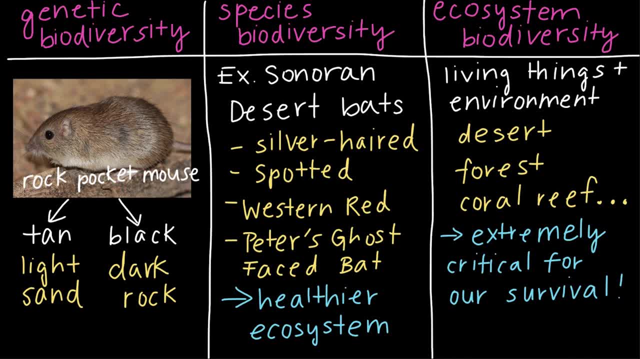 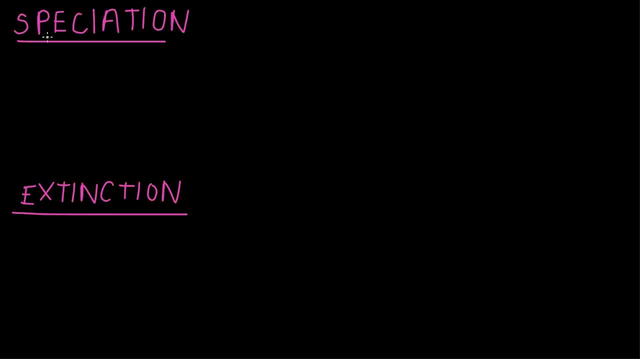 reasons. Now, biodiversity doesn't remain constant, So we can think of biodiversity as something that can change over time. Now the important thing to remember is that speciation increases biodiversity, while extinction decreases biodiversity. So let's talk about speciation. 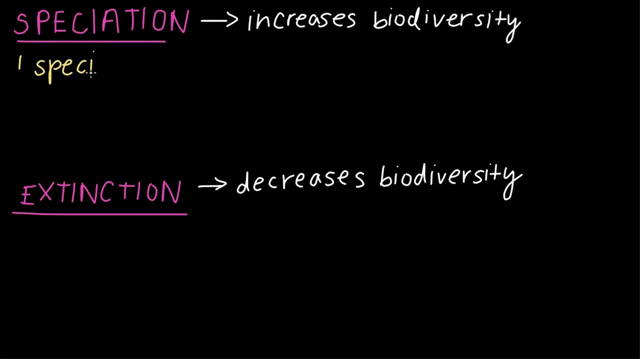 first. So speciation happens when one species evolves into another species. So if you're looking for a species that evolves into two or more species over time- and you might have heard or seen something that looks like this- and I'll draw it out right here to the right, and this is just a: 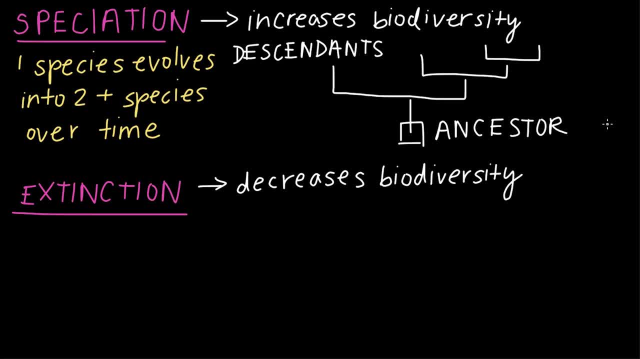 very simple speciation model or a phylogenetic tree. So we have here a common ancestor that branches off into different species over time- this arrow representing time, or T for short- and it's speciation events like these that have led to the biodiversity that we see on Earth today. 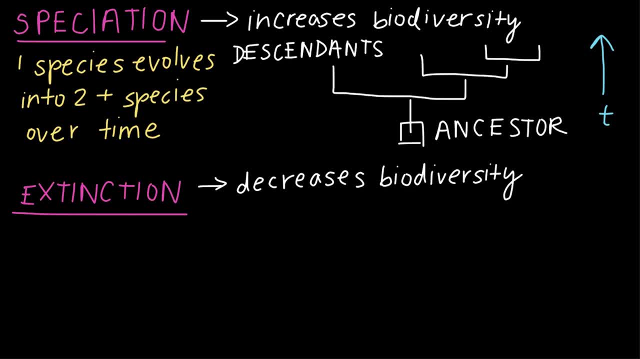 On the flip side, we have extinction, which causes biodiversity to decrease, And what we mean by this word extinction is that a species or population of living things dies off completely. So notice that it can happen on different levels too. For example, if a population goes extinct. 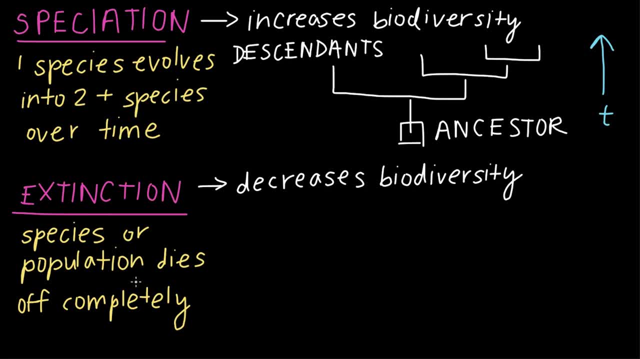 then we no longer have the genetic variants in the gene pool or the set of genes for a particular species. But if a species went extinct entirely, then that species is no longer in the gene pool. So if a species went extinct entirely, then that species is no longer. 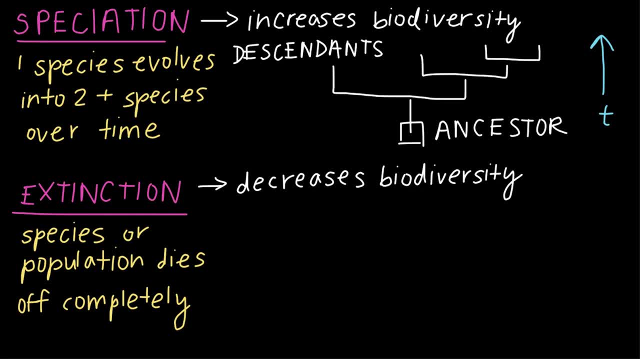 there to fulfill its unique role or its ecological niche. So you might have heard of the dodo bird, which is a species that actually went extinct way back in the 1600s. So some of the major causes behind the dodo bird's extinction include overhunting, habitat loss. 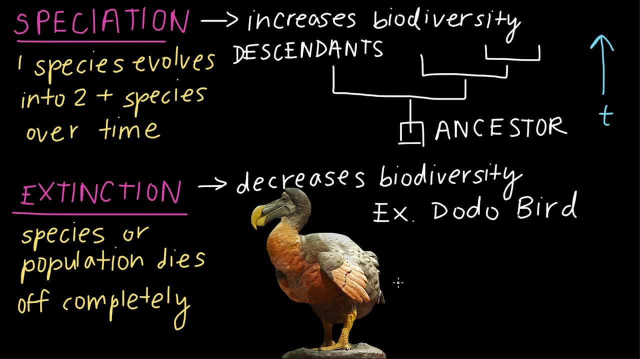 and competition with some newly introduced species. And, unfortunately, the last dodo bird was reportedly killed in 1681.. And even though we can't enjoy the presence of dodo birds, we can't enjoy the presence of dodo birds anymore. learning about this extinct bird actually brings up a really